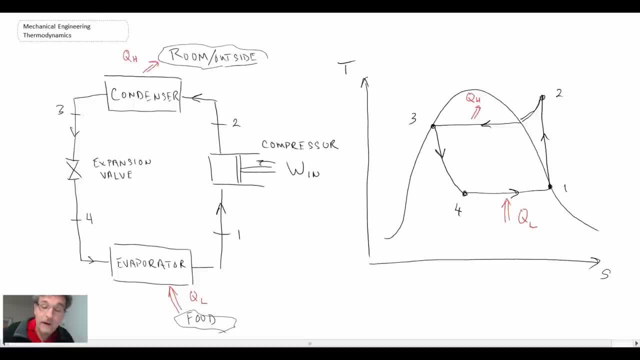 So there we can see our schematic as well as diagram for the vapor compression system And what we have remember when we were looking at the rank and I always said: start at a compressed liquid, so that would be state one. Well, when you're looking at a vapor refrigeration cycle, 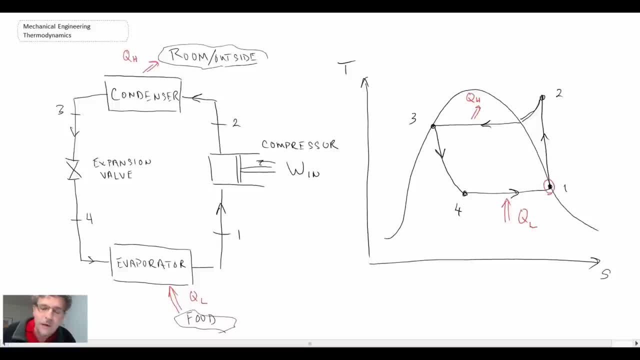 we start at the superheated line and that is at state one, which is where we go into our compressor. So we compress up, we go to state two- superheated fluid- and then we go into the condenser. So at this point we want to be at a temperature that is 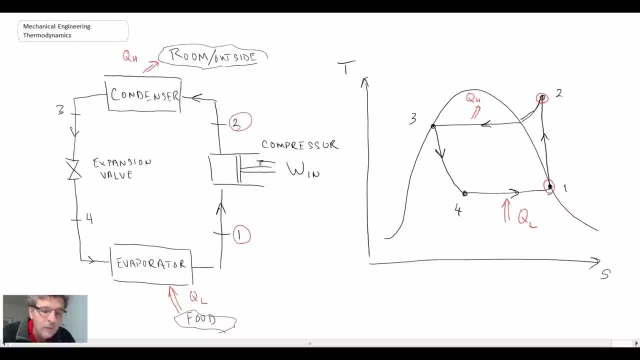 higher than our surroundings, So be that the room, in the case of a refrigerator, or outside, in the case of an air conditioning system, And we then reject heat to that surrounding environment, And that's why we want to be at a higher temperature. And through that process we then go through a 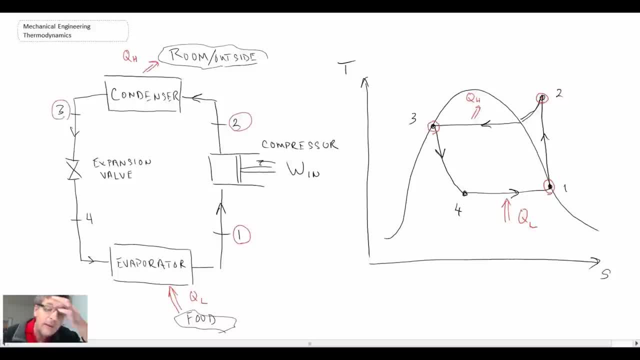 phase change operation, taking us to state three. So there we become a compressed liquid. We then go into a throttling or expansion valve and that is basically a process whereby we reduce the pressure. We model that as being a constant enthalpy process And we'll see that later on. That takes us to 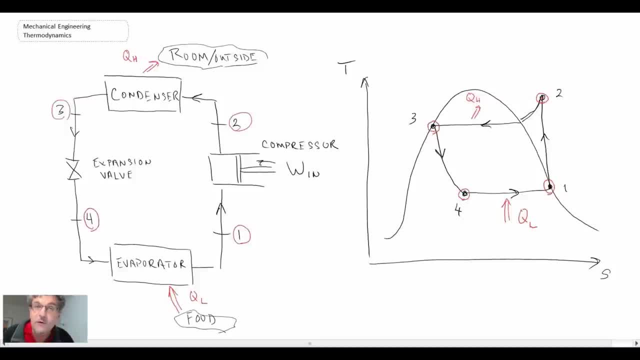 state four, And at that point we then go into whatever space we're trying to provide the cooling to and we absorb thermal energy from that space, Be it your refrigeration, so your refrigerator in your house or the space that you want to have air conditioned. 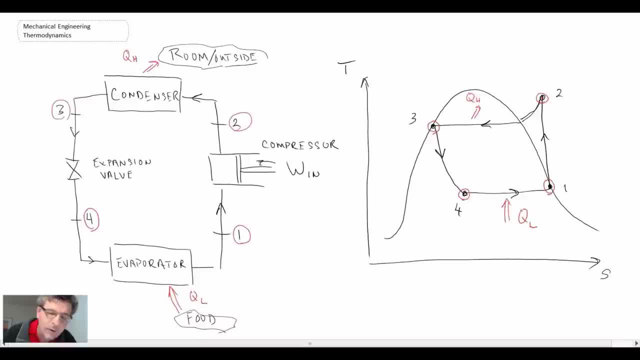 And through that process process we go through a boiling process, which we refer to as being evaporation, and through that evaporation process, what happens then? we come back to state one and repeat the cycle again. so that is refrigerator. what we're going to do now. we're going to take a look at a video, a couple of 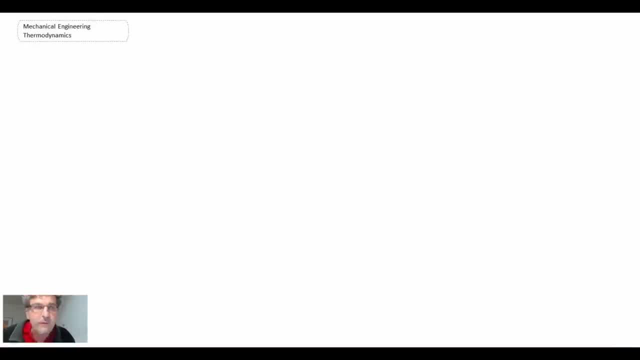 clips of an old refrigerator and a new refrigerator and you'll see the change in design. the new refrigerator is a little more compact, but we'll begin with the old refrigerator. so let's take a look at that now. and so what? we see the compressor on the bottom. there is the hot refrigerant going. 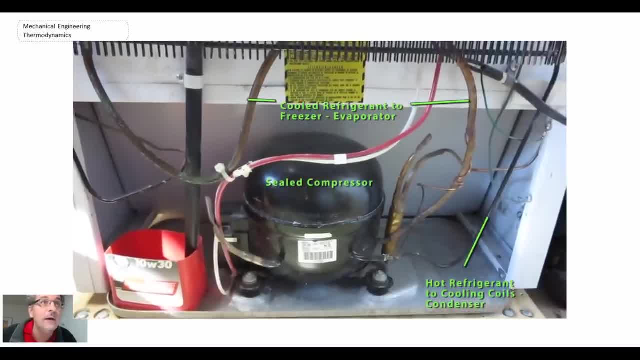 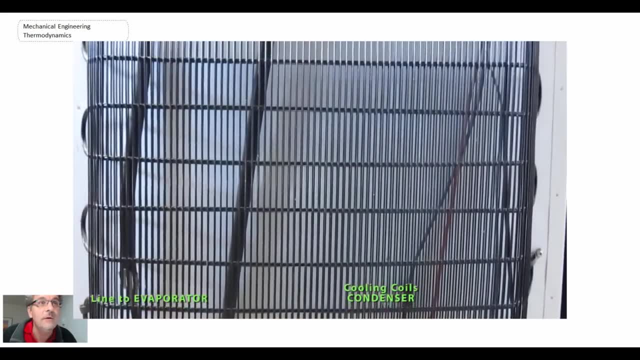 up to the cooling coils which are mounted on the back. those are the condensers. and then there's another tube on the left. there, the tube on the left is going up to the evaporators that will flow into your freezer and provide cooling for your food. the cooling coils on the back. it's. 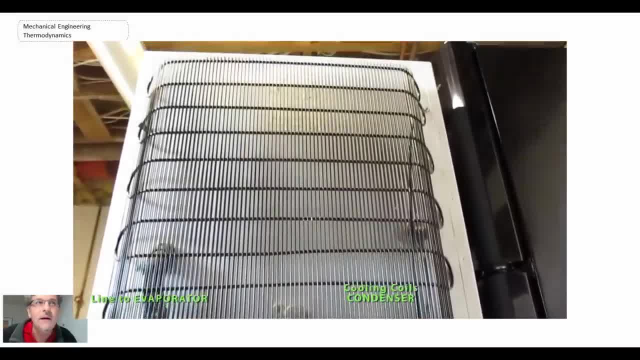 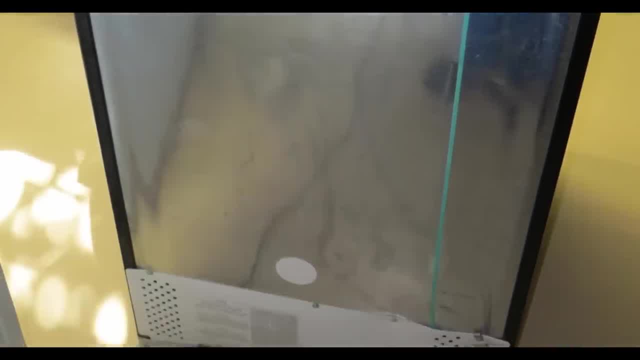 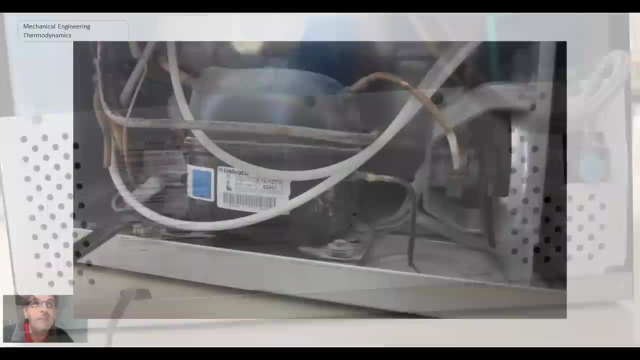 basically just a copper pipe with it's probably a steel wire that's connected to it that assets fins for for heat transfer. this is a modern refrigerator. notice there are no coils on the back. everything has been compactly placed underneath so it's a lot cleaner. you don't get dust buildup. so there's our compressor in the 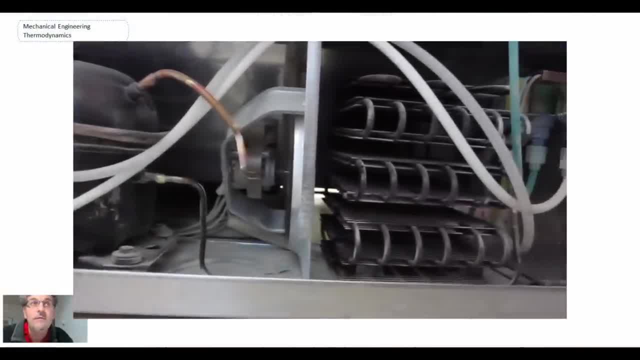 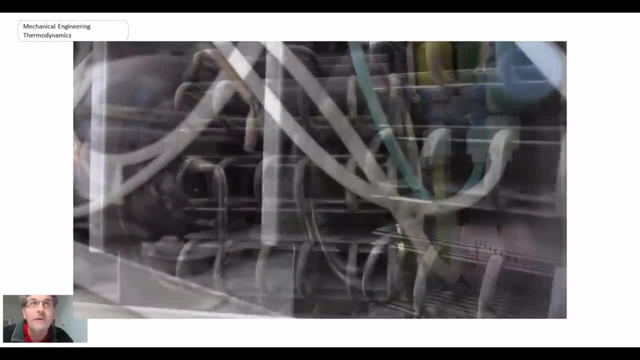 middle is a fan which actually causes forced convection, and that comes over our cooling coils, our condenser. you see the condenser is neatly compacted in the bottom of the unit, no longer on the back, and then you can see the line coming out of the compressor, just like we had. 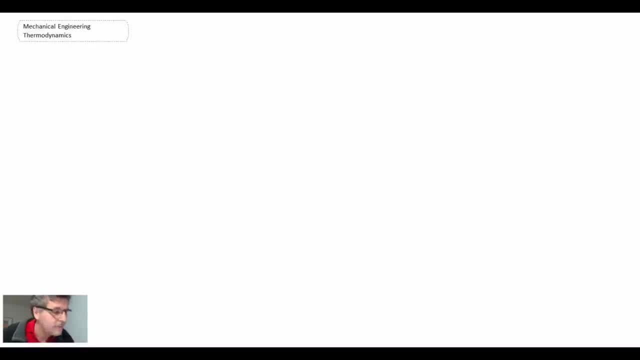 an old refrigerator and a new refrigerator. they basically do the same thing, except the new design is a little more compact and cleaner. so the last thing that I want to mention about the vapor compression systems is that when we're looking at a real one in an actual cycle, we will deviate a. 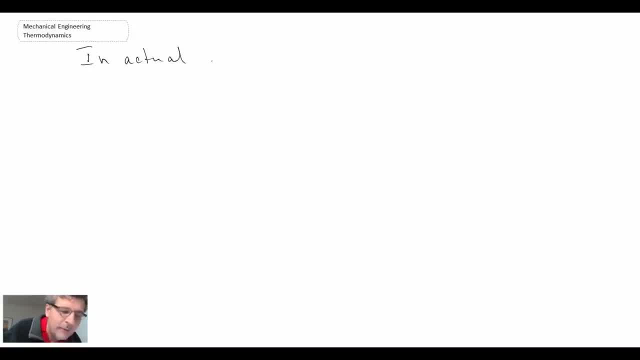 little bit from what we've looked at and that was kind of an ideal representation of the vapor compression refrigeration cycle. so those are the differences that we would find in a real world system. let's write out our TS diagram again and we'll look at those points. so we start at saturated vapor line that state one going to. 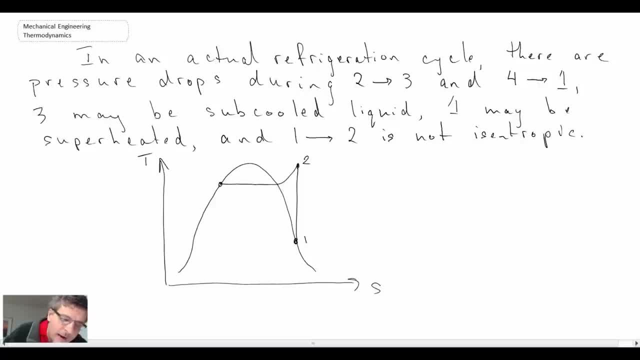 the compressor. then we come back to the liquid region, go into the throttling valve, taking us to four. so that is the representation that we have for an ideal cycle. now, in reality, what we're saying is that you'll have some deviations here. one is that you're going to 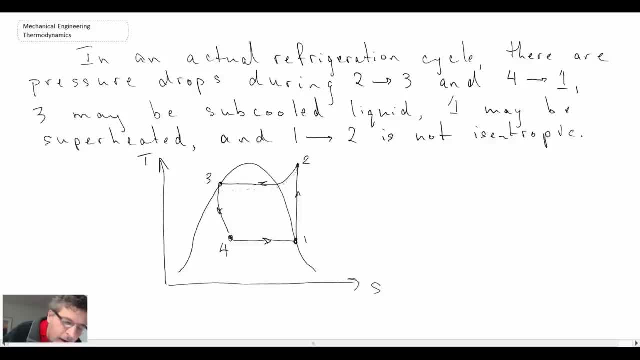 have pressure drops going from two to three and consequently the pressure will drop there. you'll have a drop in pressure here and that may take us into a sub-cooled liquid region for state three and superheated for state one. and the other thing is that when we go through the compression process itself, it may not be isentropic.